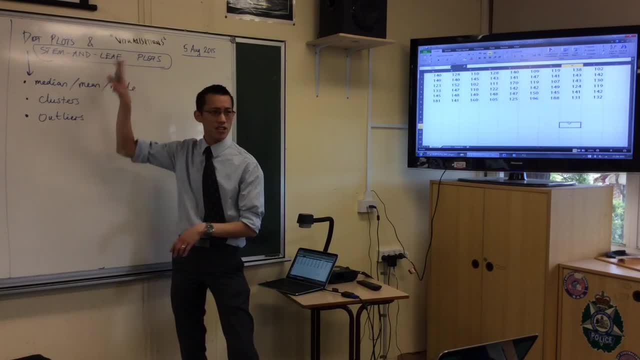 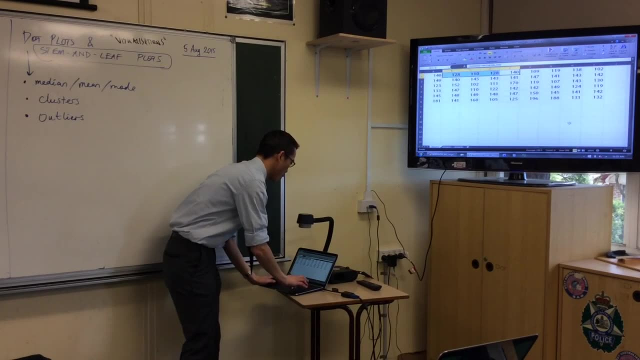 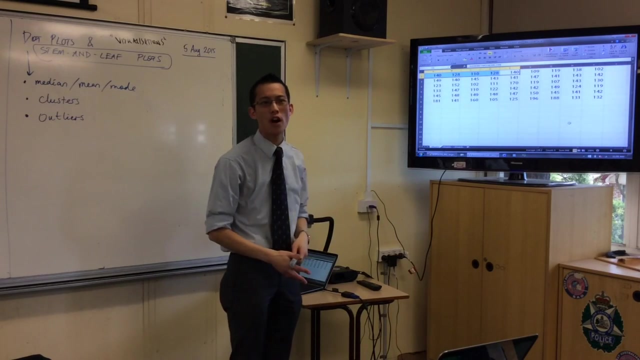 Okay. Now, when you get these visualizations, they're really useful when you have large amounts of data. If all you've got is, say, these five guys at the top- one, two, three, four, five- you don't need to draw a graph for that. You just look at the numbers and it's easy to get in your head. But when you look at that it's like, oh, it's a bit overwhelming. If I can visualize it, I can understand it better. okay, So here's the first thing that we're all going to do: Let's get this data. Let's get it in some order- It's completely random at the moment. okay, 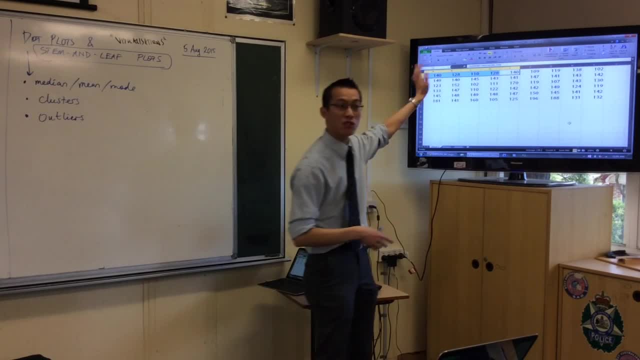 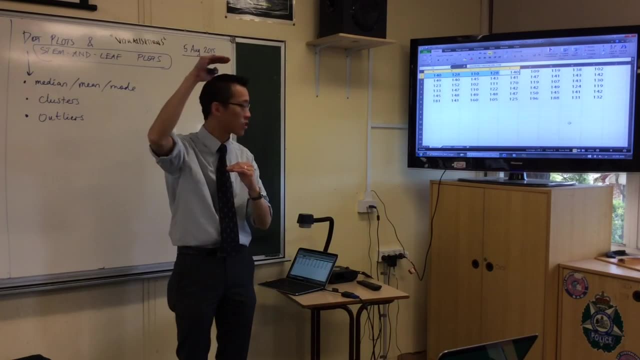 You could put it just in like numerical order. You could sort it okay. But to help you do that a bit quicker, I want you to notice what's the range of the data Like what's the lowest score you can see and what's the highest score. 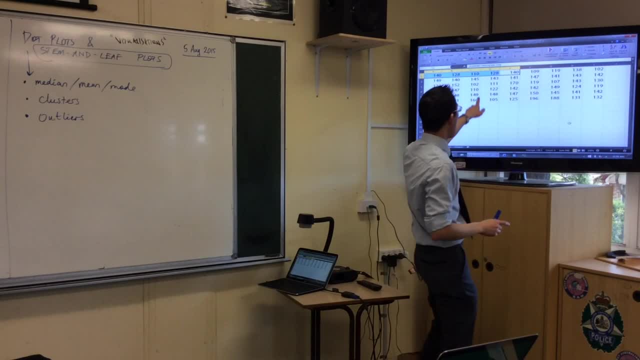 One hundred and two. One hundred and two, One hundred and two. Okay, I can hear. one hundred and two sounds like it's the smallest, okay, and it looks pretty good. I don't see one hundred and one. I don't see a hundred. I don't see any two digits. 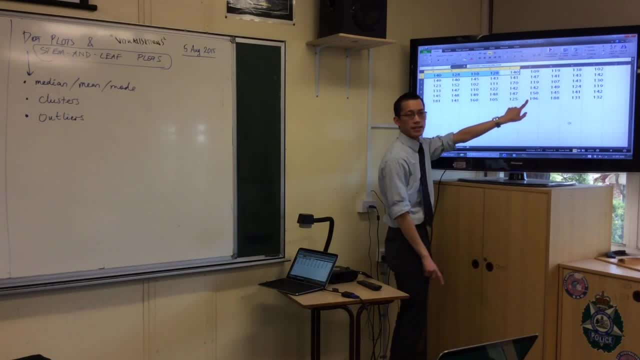 And what's the biggest score? One hundred and eighty-eight, One hundred and ninety-six. It looks like one hundred and ninety-six. One hundred and ninety-six, One hundred and ninety-six. Do we have anything beating that? No, It looks pretty high. 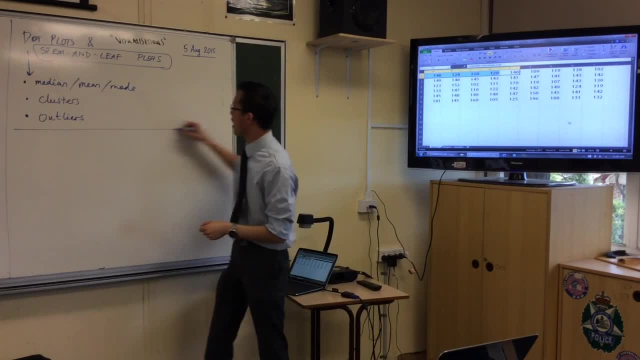 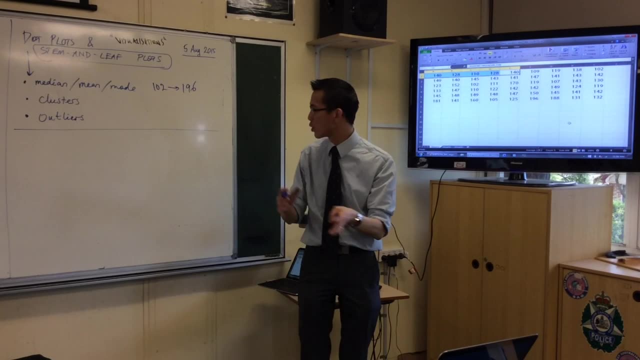 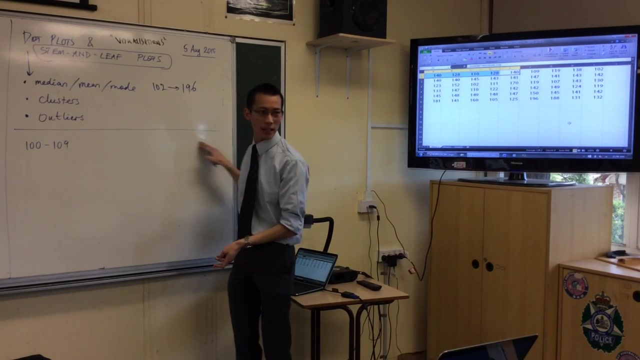 Okay, So, being that we have data from one hundred and two all the way up to one hundred and ninety-six, okay, What we could do is sort of group this, We could group this. We could have, like all of the numbers from one hundred to one hundred and nine here, right, We can group them. 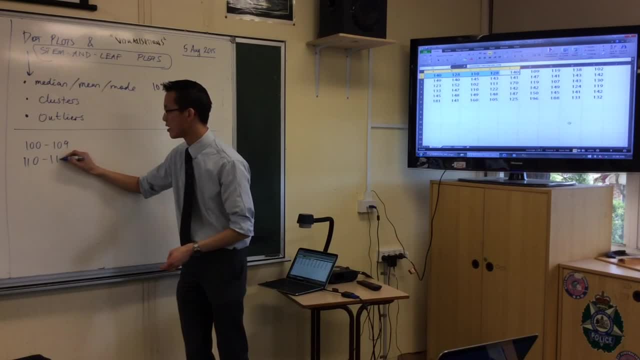 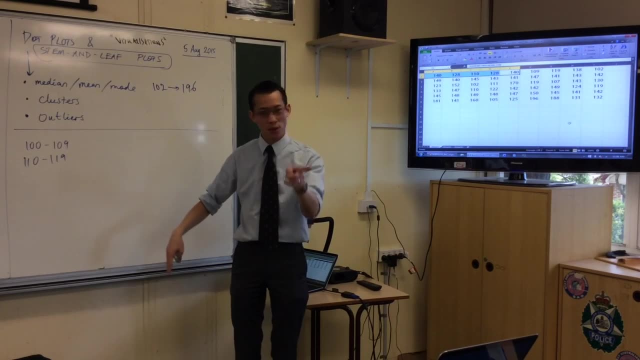 We can have all the numbers from one hundred and ten to one hundred and nineteen. Group them all here, Okay. All the way down I'm going to have a whole bunch of different sets, Okay. So that's what I'd like you to start by doing. 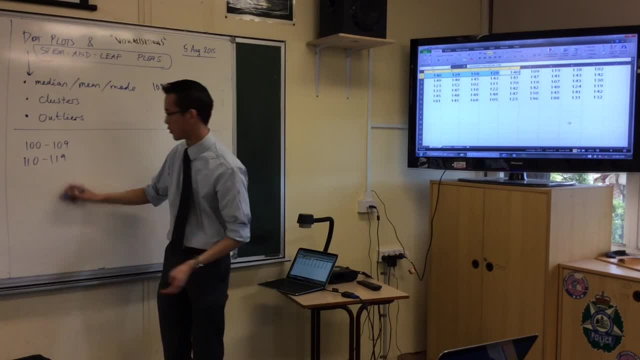 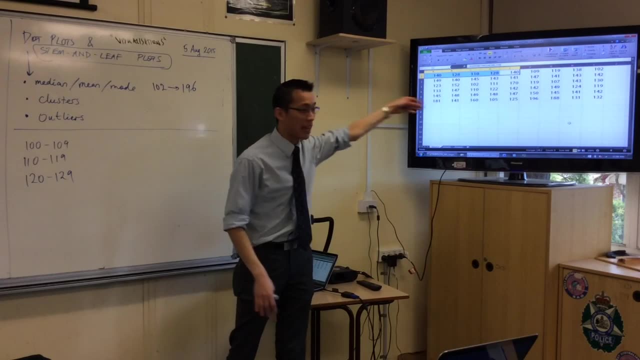 I've got some categories for you. I'll finish this list off, but you can finish it off yourself too. Let's group these scores in these groups and then we'll be able to see some patterns here. Okay, Look carefully. If you didn't miss any, I'll leave that on the screen. 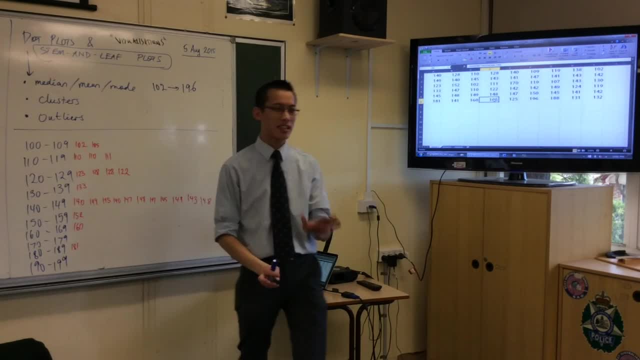 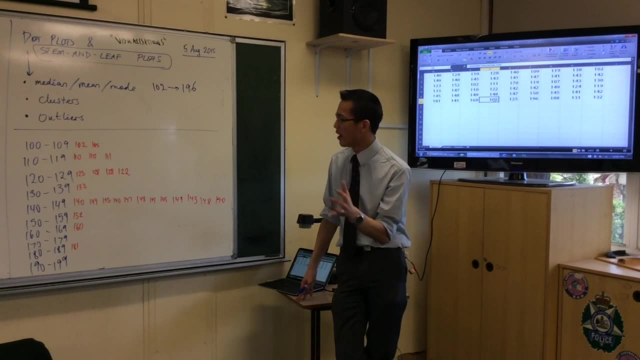 Okay. Okay, Because there's a lot of data there, It takes a long time. You're starting to sense man. this is not the most efficient way to do this right, But surely there's got to be a better way. 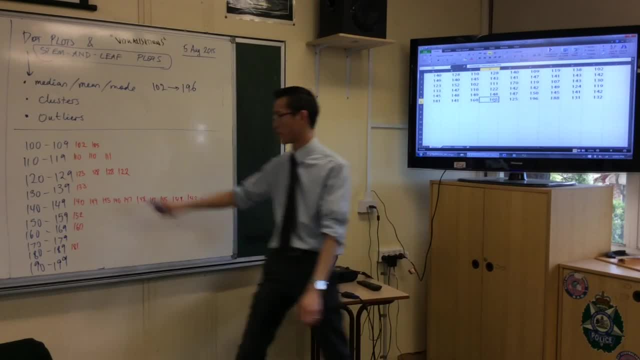 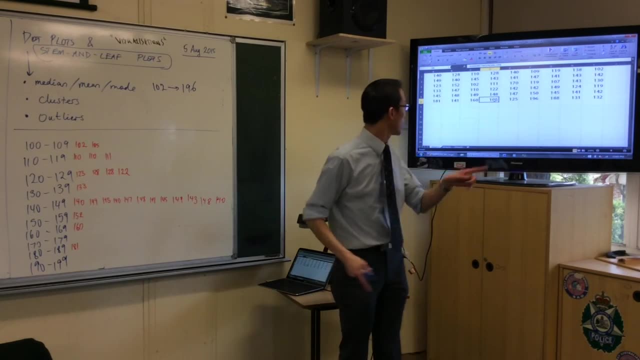 I do want to get these in order, And you know it would certainly be harder to try and put them in completely random order, with no categories. But this is Tiduson and it takes a lot of space. I mean, if you notice what I'm doing, I'm going down the columns right and then I'm just filling them in. 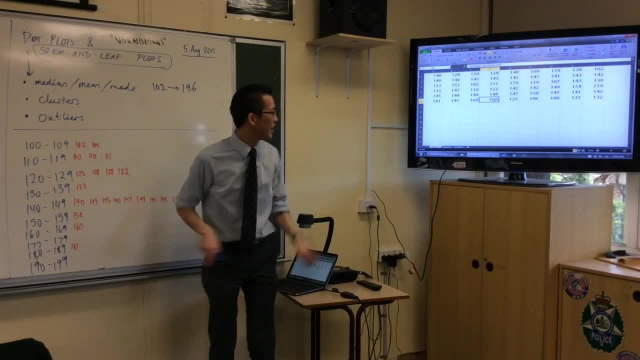 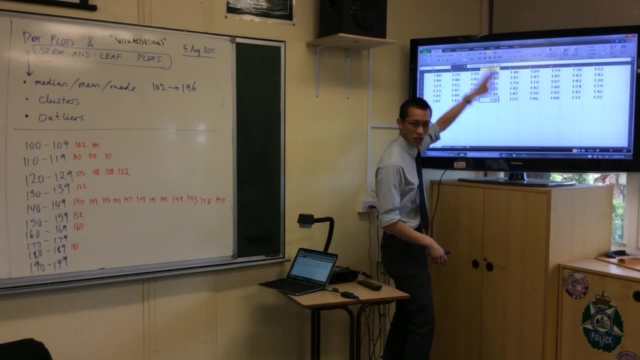 The reason I'm doing that, rather than looking for all of these ones and then all of these ones, is I don't want to miss any Right. So if I know I'm going down here, I'm not going to accidentally say, whoop, forgot a score. 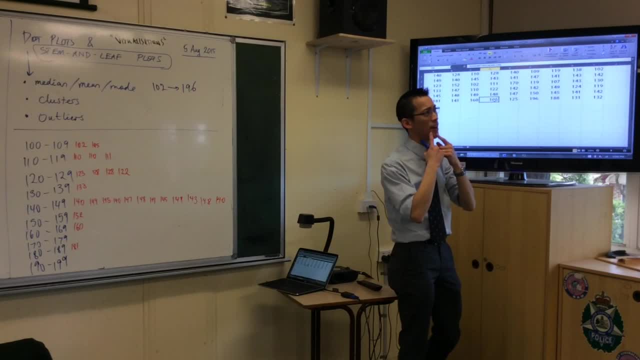 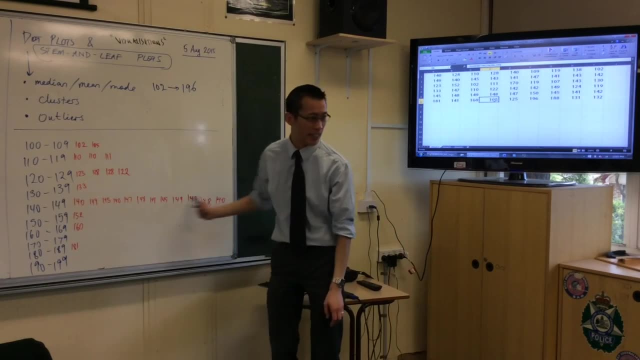 I'm just going to go through in a loop- Sorry, What's the loop? In a methodical way, So I'm not going to miss any That make sense. But have a look at this right, Look at this line in here in particular, right? 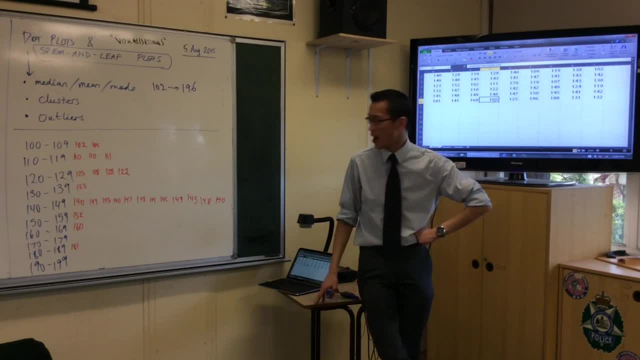 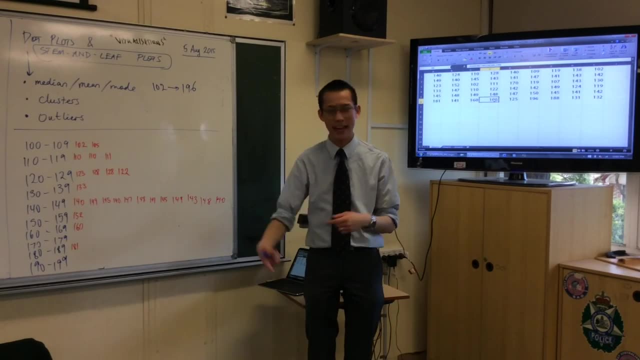 This is taking me forever And it's wasting loads of space. I'm writing 140,, 149,, 140.. I'm writing the 1 and the 4 over and, over and over again, And every score in this category is going to start with a 1 and a 4, right. 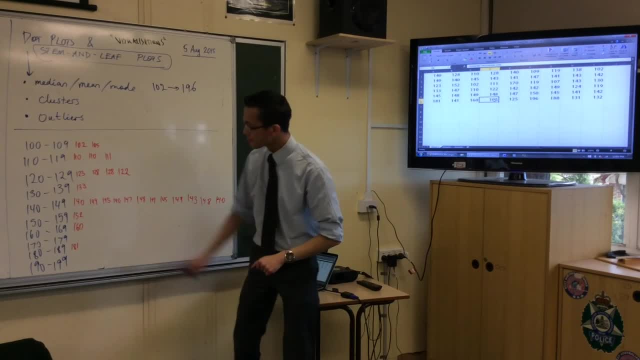 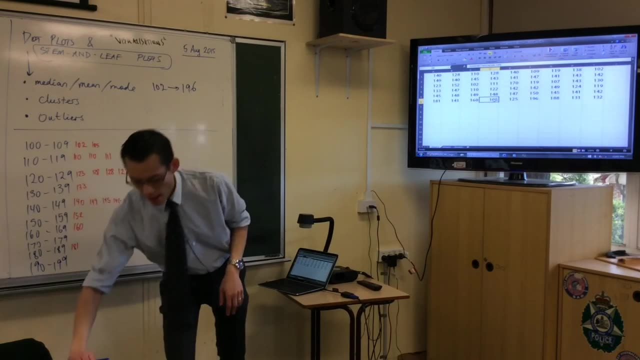 So here's a better way to do this, Being that all of these scores are going to be in order. All of these scores have 1 and 4 in common, And all of these scores have 1, 3, 1, 2, 1, 1,, etc. 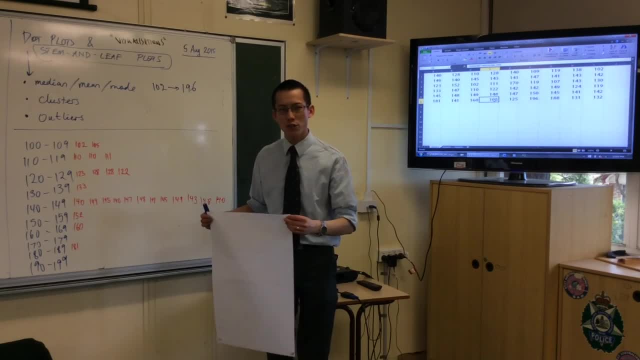 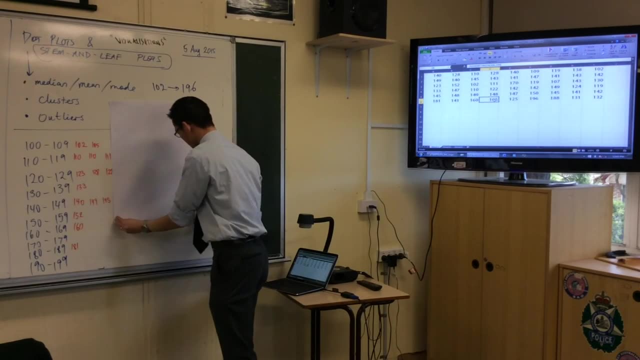 Underneath where you started doing this. I'm going to ask you to make another plot, But it's going to start off a little bit different. We can finish this one later, But this one is going to be much better. So here's what we're going to do. 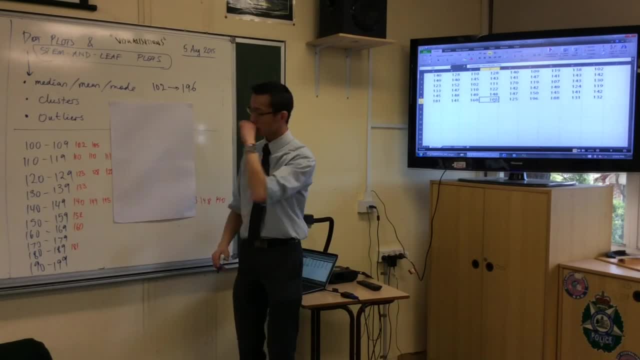 I want you to, with your ruler, if you've got one. If you don't have one, you can get one later. We're going to rule a couple of lines to make what we call a stem and leaf plot, And you'll see why it's called a stem and leaf plot in a minute. 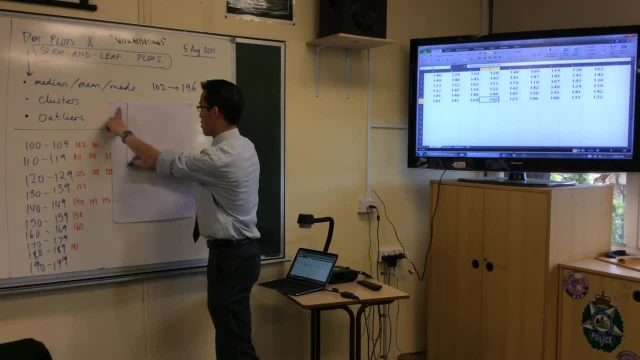 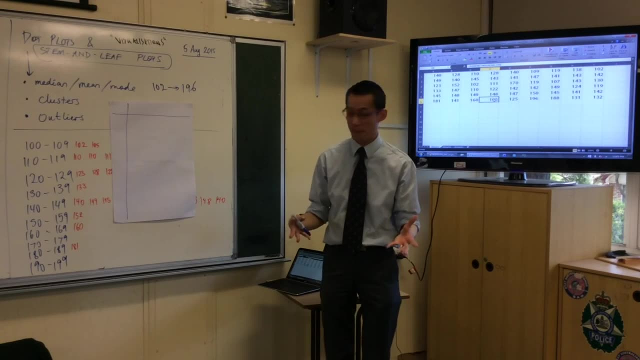 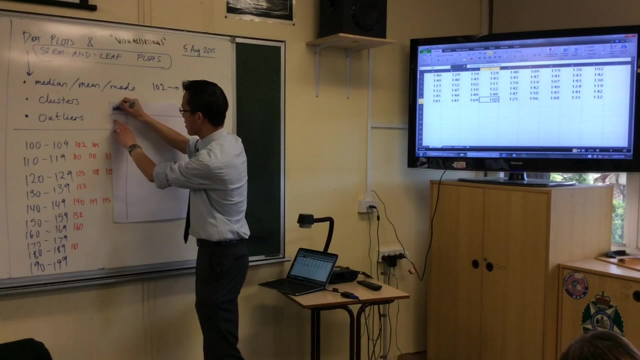 The couple of lines go like: so One down this way. So this stem and leaf plot is made of two parts, unsurprisingly: The stem and the leaf. So we've got a stem over here And what I'm going to get is a bunch of leaves over here. 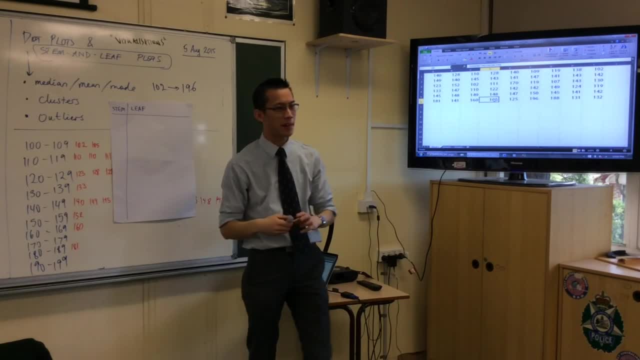 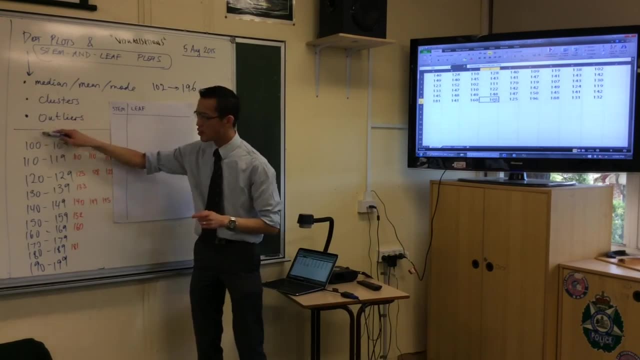 And I'm going to explain what those are in a second. So remember, here are my categories right: 1, 0, 0, 1, 0, 1, 1, etc. These all start with 1, 0. 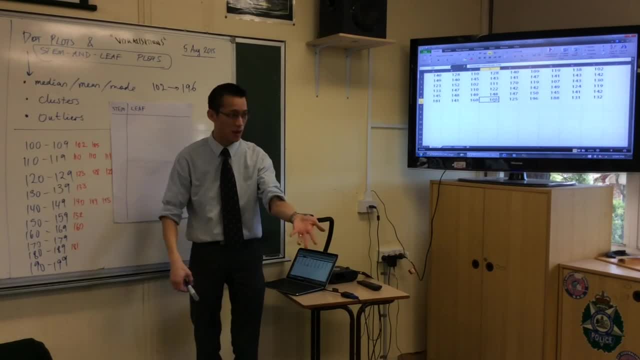 These all start with 1, 1.. All start with 1, 2,, etc. So the stem is how your numbers begin. So I'm going to call this 1, 0, 1, 1, 1, 2,, 1, 3.. 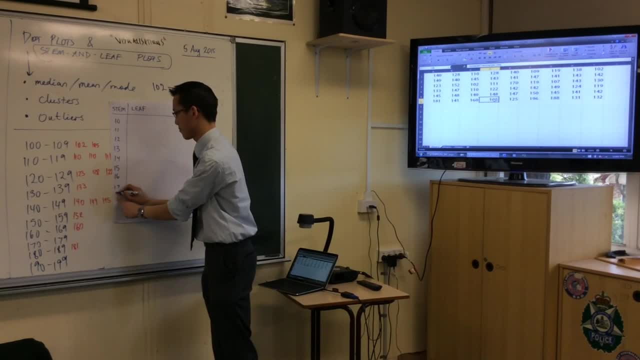 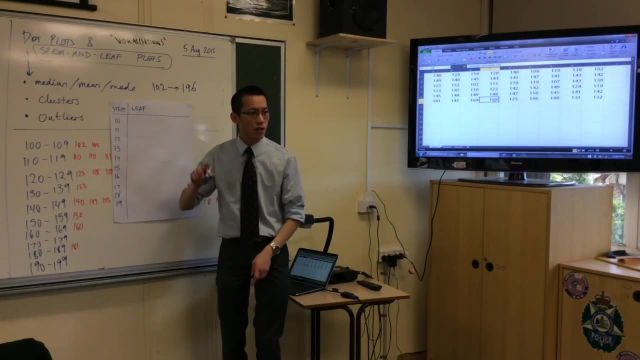 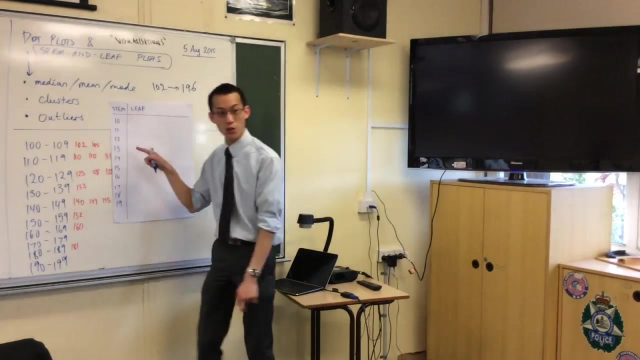 You get the idea. OK, You with me so far. So here are going to be all the numbers that start with 1, 0.. Now you notice I've already got some numbers here. OK, 2, 102, 105.. 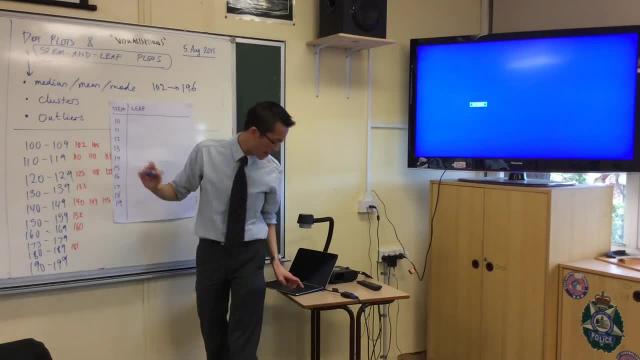 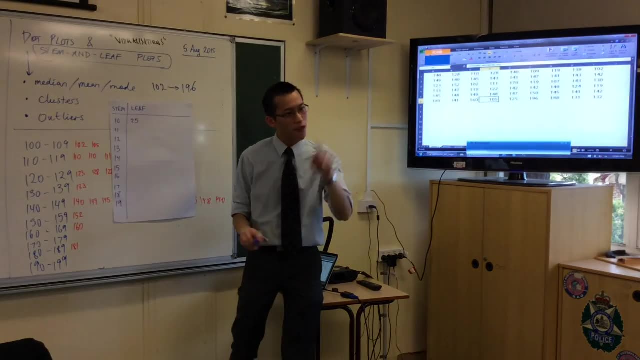 So all I write is: and just note- I'm going to put these all the same distance apart. I'm going to write the 2 and then the 5.. I'm going to put them right next to each other, The 2 and the 5,. they symbolize 102.. 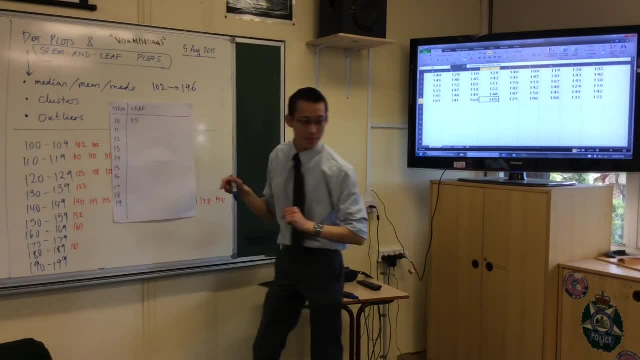 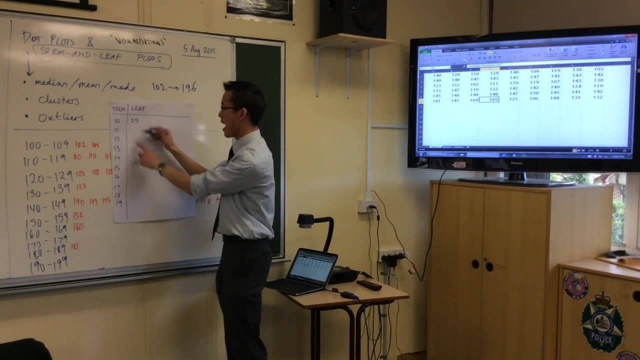 105.. OK, Yes, question No. I'm going to put them right together. OK, and you'll see it like this: Here I'm going to have 110,, 110, 111.. I'm going to have a few more scores going this way. 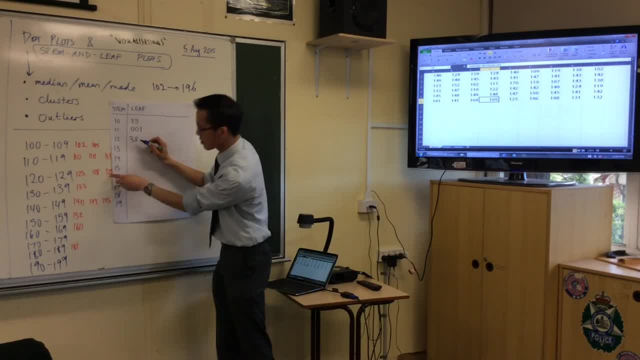 123,, 128.. Can't see 8.. 128, etc. What's this next one going to be here? It's just the 3, 133.. I've got a whole bunch here: 0,, 9,, 1.. 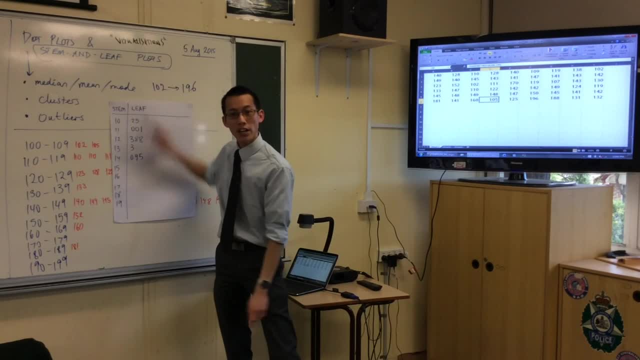 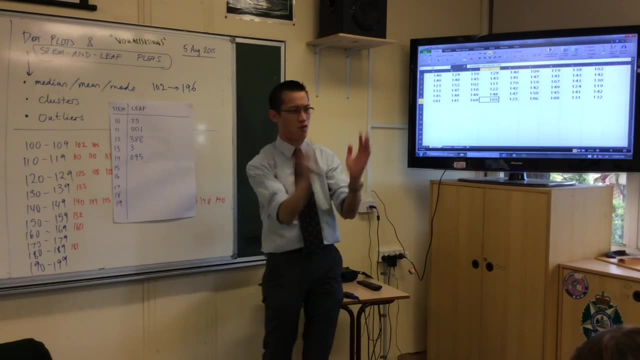 OK, now here's what we're going to do. Two things. Number one: we're going to complete this all together. Secondly, I want you to note right, See how I'm putting just the numbers. I'm just jamming them right together. 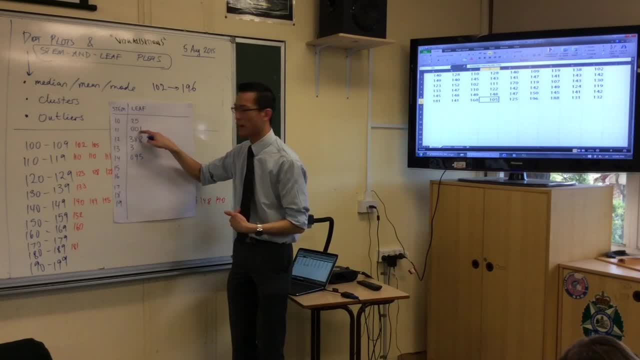 OK, That's because I know that each one of these is what I call a leaf. It's its own number. This is not like 388, for instance. OK, I set up this so that I know that's 123 and 128 and another 128.. 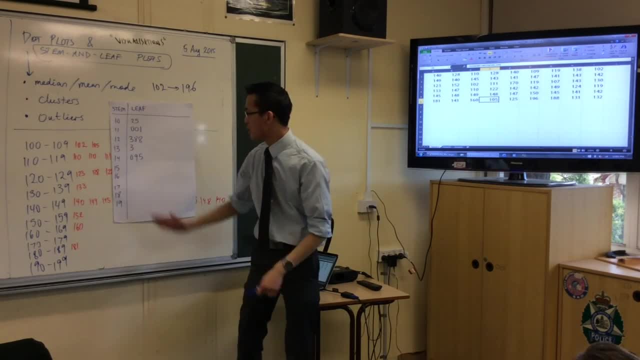 OK, So that's how I'm reading it. You'll notice I've evenly lined up my numbers right. These numbers all line up. These numbers all line up, And you'll see why once we finish this plot. that's really important. 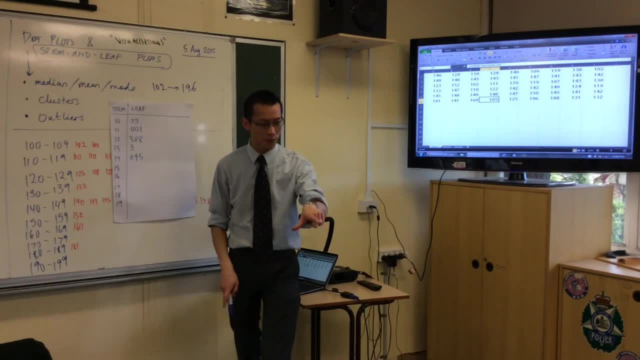 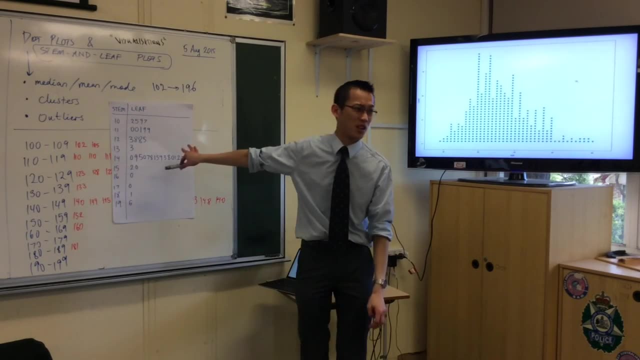 OK. So you've got this set up. I'm going to finish it, and you can finish it as well. Let's create this stimuli plot. I'm almost done. I'm almost done. Let's say two things. Number one: this is not in order yet.